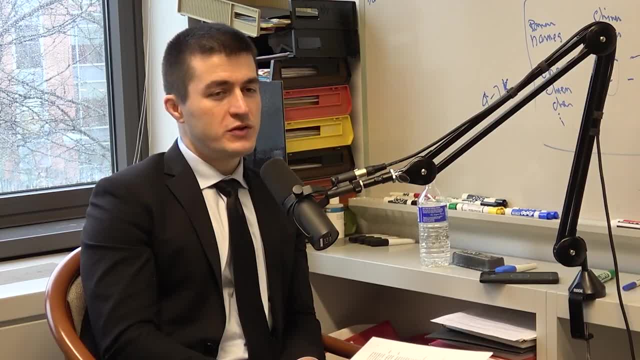 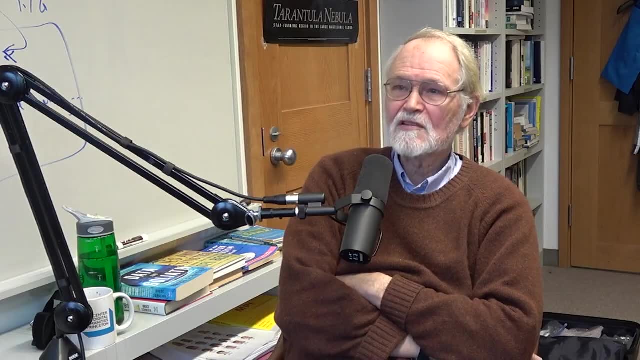 So everybody had their own assembly language, And assembly languages have a few commands, additions, subtraction, then branching of some kind. if then type of situation Right, They have, exactly in their simplest form, at least one assembly language, instruction per instruction, in the machine's repertoire, And so you have to know the machine intimately to be. 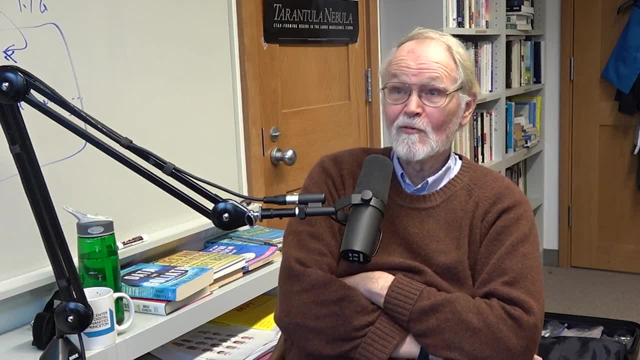 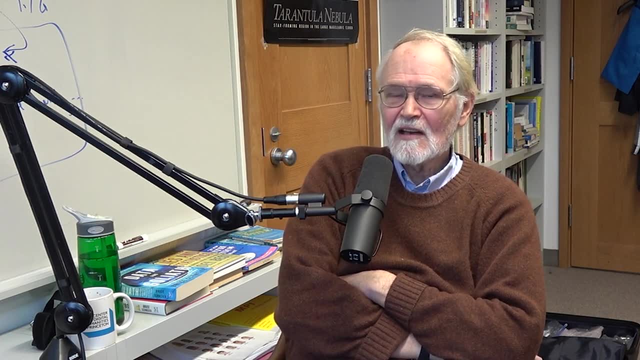 able to write programs in it. And if you write an assembly language program for one kind of machine and then you say, geez, it's nice, I'd like it in a different machine, Start over, Okay, So very bad. And so what happened in the late 50s was people realized 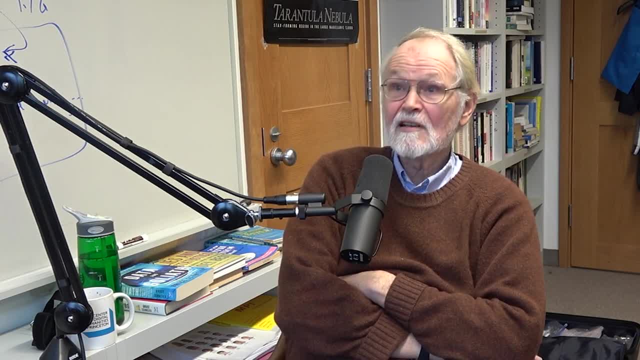 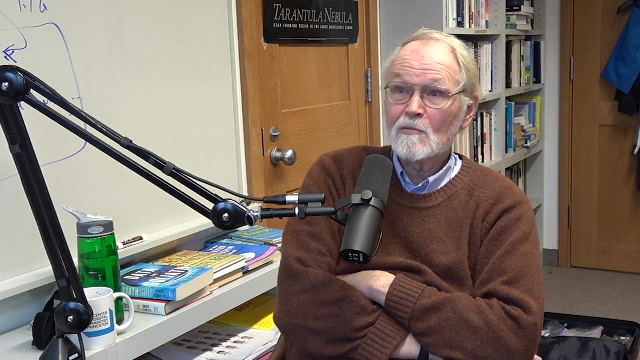 you could play this game again and you could move up a level in writing or creating languages that were closer to the way that real people might think about how to write code, And there were, I guess, arguably three or four at that time period. There was Fortran, which came from IBM. 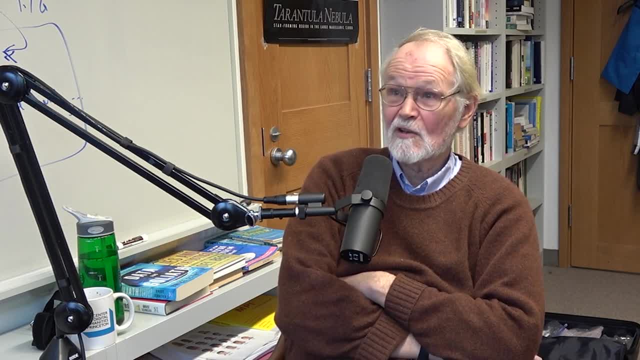 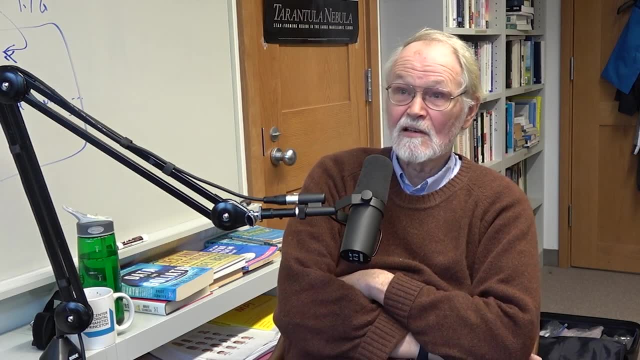 which was formula translation, meant to make it easy to do scientific and engineering computation. I didn't know that. I didn't know that Formula translation. That's what it stood for. There was COBOL, which is the common business-oriented language that Grace Hopper and 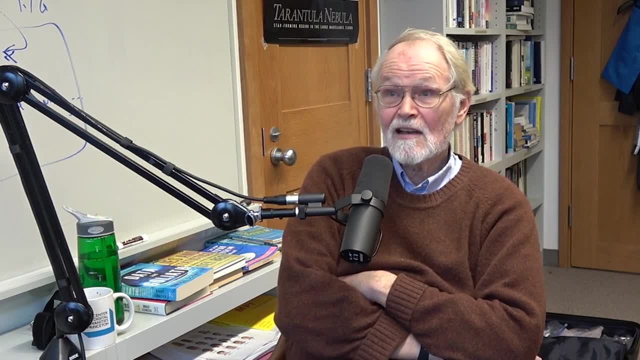 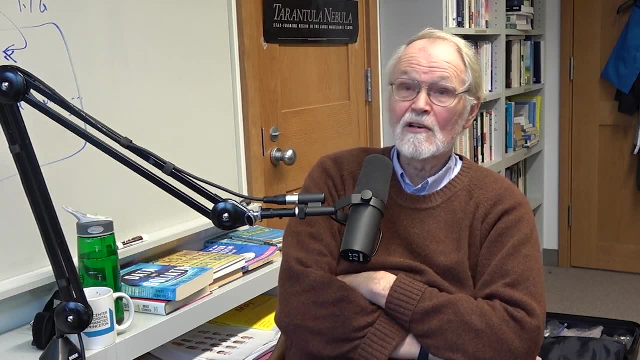 others worked on, which was aimed at business kinds of tasks. There was ALGOL, which was mostly meant to describe algorithmic computations. I guess you could argue BASIC was in there somewhere- I think it's just a little later- And so all of those moved the level up And so 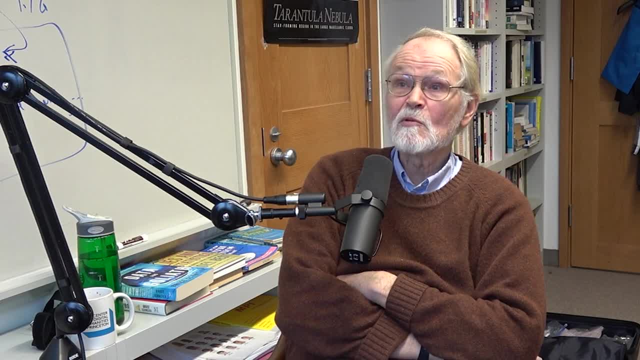 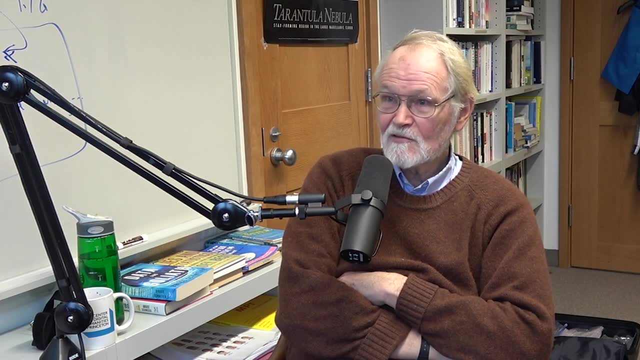 they were closer to what you and I might think of as we were trying to write a program And they were focused on different domains: Fortran for formula, translation, engineering, computations, let's say COBOL for business, that kind of thing. 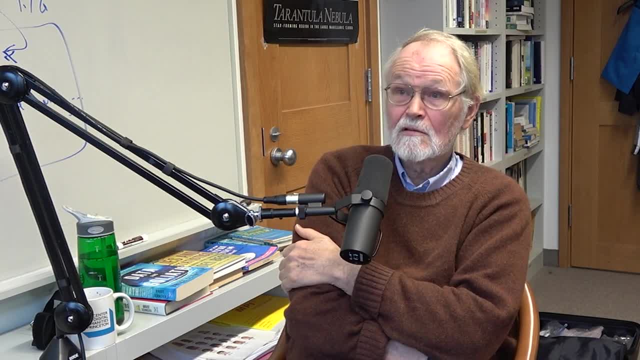 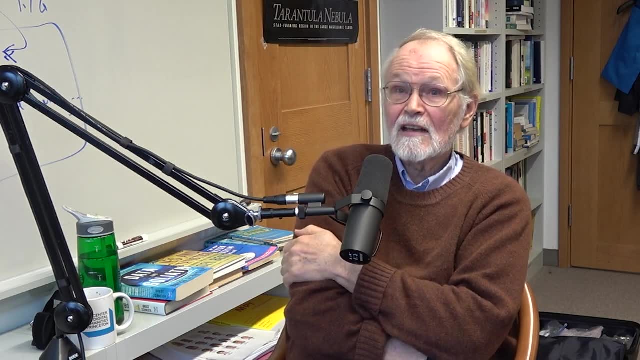 And still used today, at least. Fortran probably. Oh yeah, COBOL too COBOL. But the deal was that once you moved up that level, then you- let's call it Fortran- you had a language that was not tied to a particular kind of hardware, because a different. 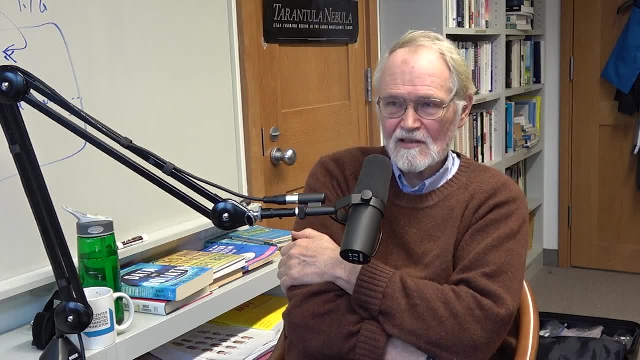 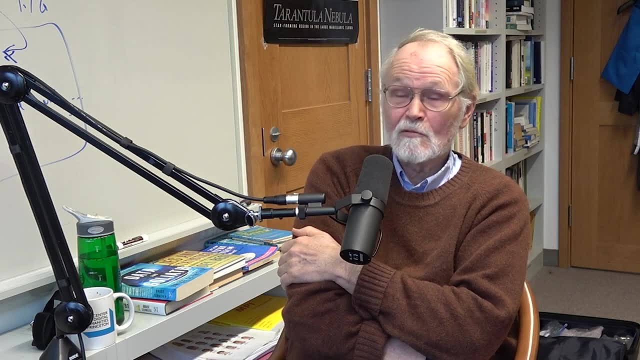 compiler would compile for a different kind of hardware, And that meant two things: It meant you only had to write the program once, which was very, Very important, And it meant that you could, in fact, if you were a random engineer. 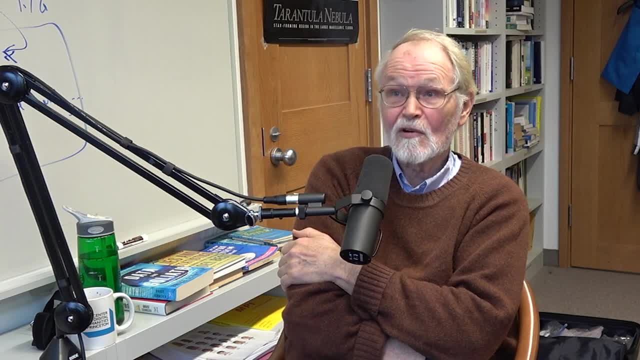 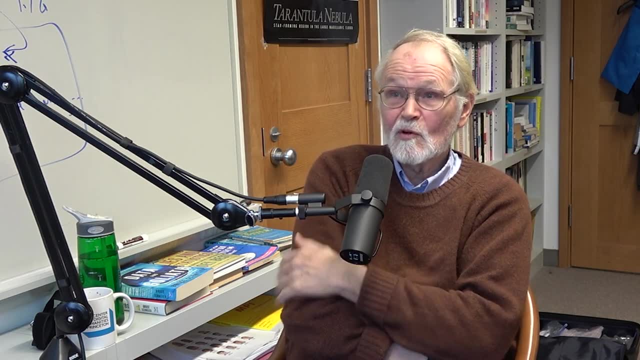 physicist. whatever. you could write that program yourself. You didn't have to hire a programmer to do it for you. It might not be as good as you'd get with a real programmer, but it was pretty good. And so it democratized and made much more broadly available the ability. 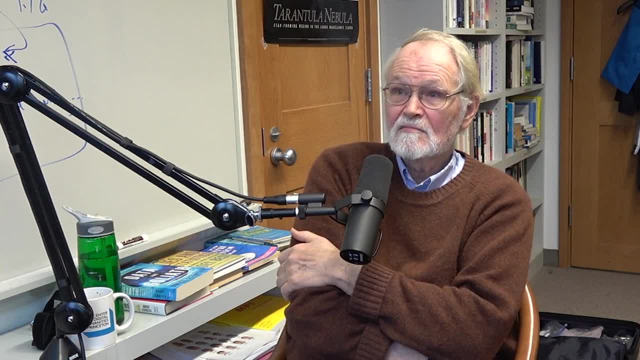 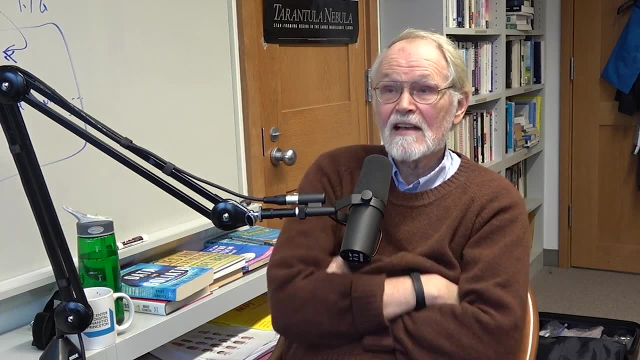 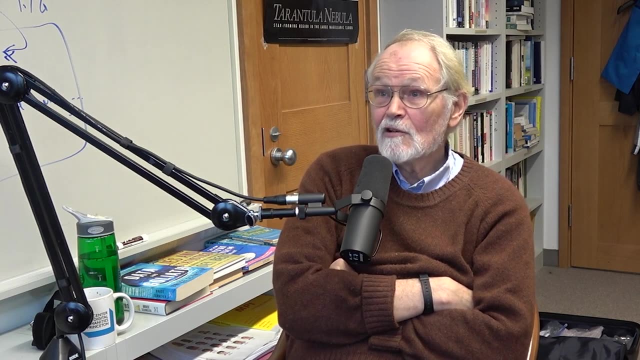 to write code. So it puts the power of programming into the hands of people like you- Yeah, Anybody who is willing to invest some time in learning a programming language and is not then tied to a particular kind of computer. And then, in the 70s, you get system programming languages, of which C is the survivor. 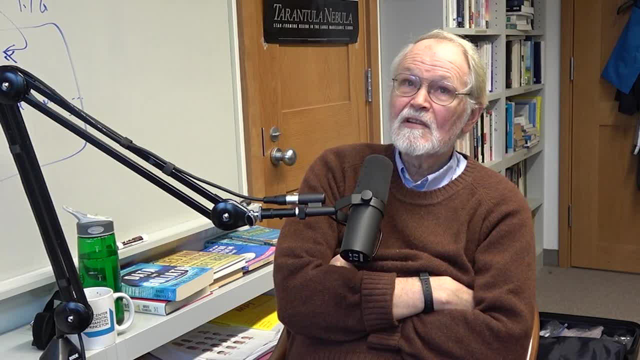 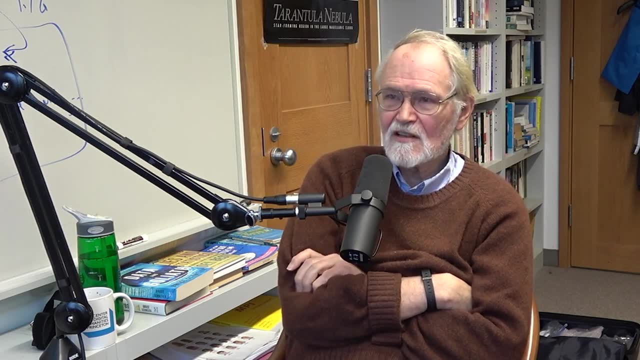 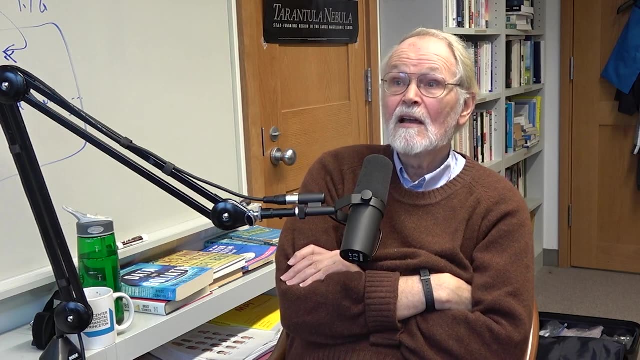 And What does system programming languages mean? Programs that Programming languages that would take on the kinds of things that were necessary to write so-called system programs, things like text editors or assemblers or compilers or operating systems themselves, those kinds of things And Fortran. 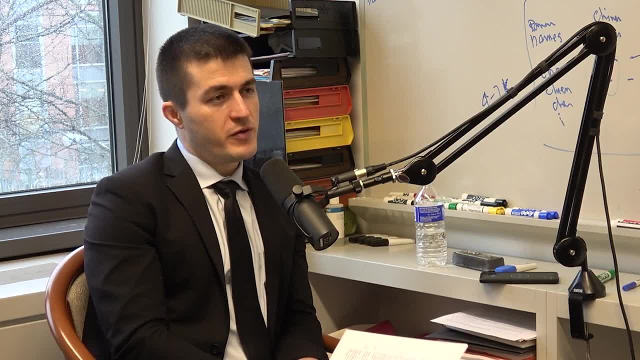 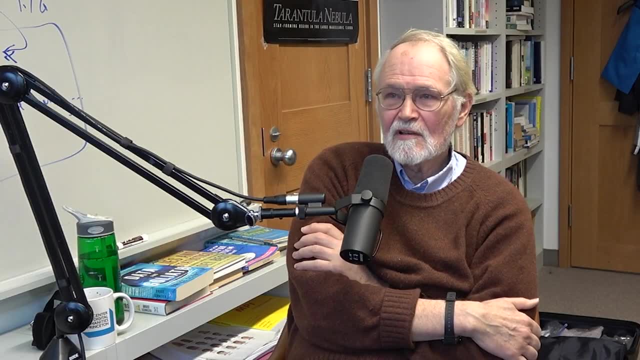 Let's be feature rich. They have to be able to do a lot of stuff: a lot of memory management, the actual Access processes and all that kind of stuff. They have to Parallel processing. It's a different flavor of what they're doing. They're much more in touch with the actual machine. 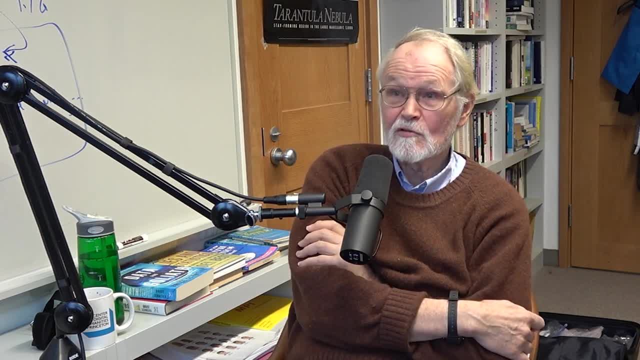 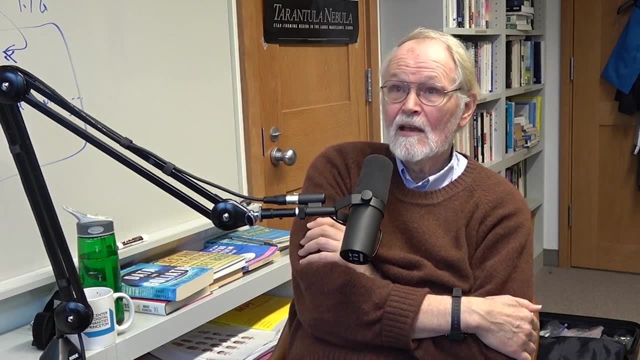 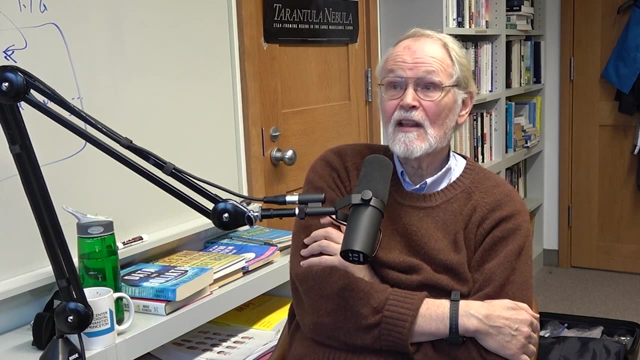 but in a positive way, That is, you can talk about memory in a more controlled way, You can talk about the different data types that the machine supports and more ways to structure and organize data, And so the system programming languages. there was a lot of effort in that in. 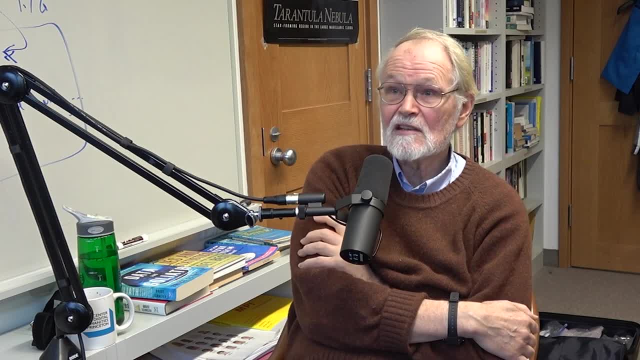 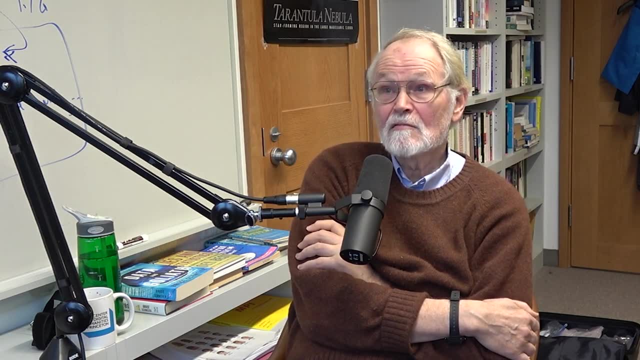 the Call it the late 60s, early 70s. C is the survivor- I think the only real survivor- of that. And then what happens after that? you get things like object-oriented programming languages, because as you write programs in a language like C, 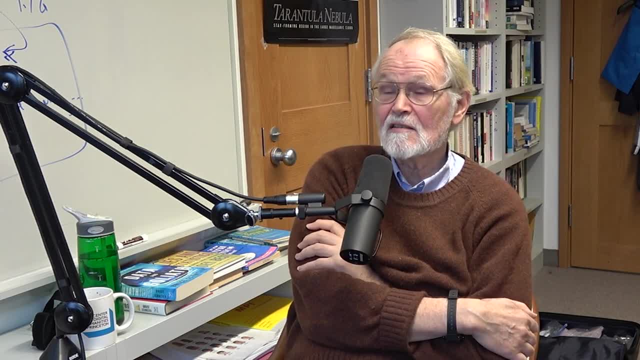 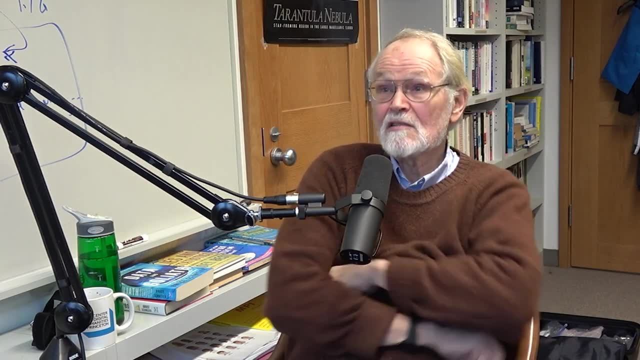 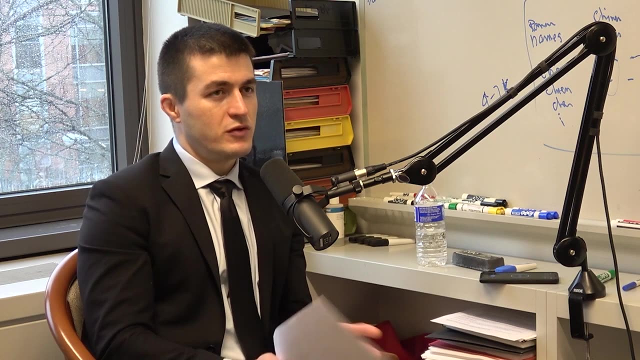 at some point scale gets to you and it's too hard to keep track of the pieces and there's no guardrails or training wheels or something like that to prevent you from doing bad things. So C++ comes out of that tradition And then it took off from there. I mean, there's also a parallel, slightly parallel- track with a 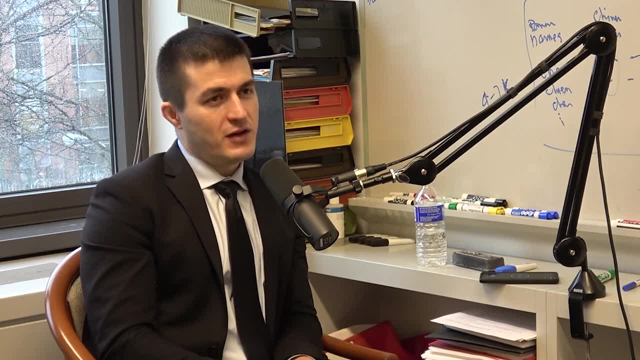 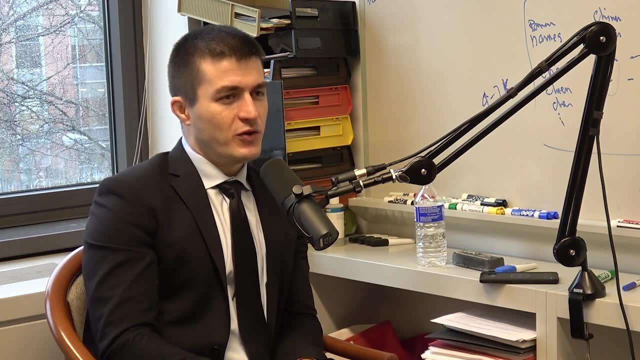 little bit of Functional stuff with Lisp and so on, But I guess from that point it's just an explosion of languages. There's the Java story, there's the JavaScript, there's all the stuff that the cool kids these days are doing with Rust and all that. 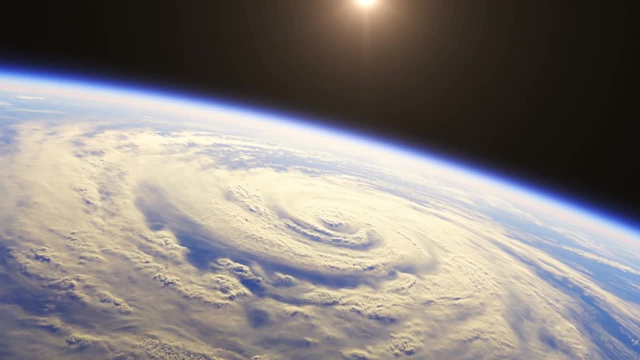 They're like: yeah, but we're not sure. There is this weird thing you can do to stuff that is not necessarily Java, And that's pride, that's where it's at, That's right. And then you get to see a lot of different things like a lot of different ways that you can do.